find the start time, So they need to arrive at the airport 16 minutes before the flight. So they're going to need to spend 16 minutes in the airport. and it takes them 15 minutes in the car to reach the airport. and they are going to need to arrive at the airport 16 minutes before the flight, So they need to. 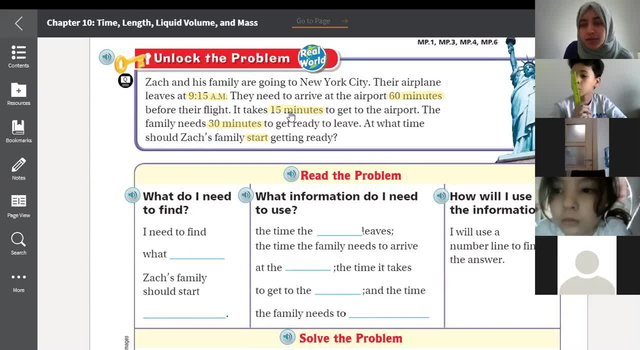 they also need 30 minutes at home to get ready, So we are going to need to add all the elapsed time to find out how much time they need before they start getting ready. So in the first part- Azza, tell me what the first part is, please. What do I need to find? 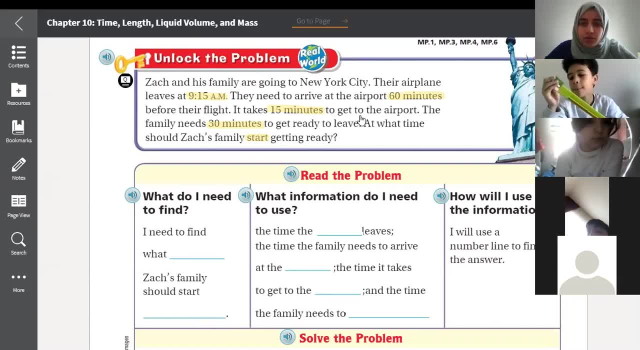 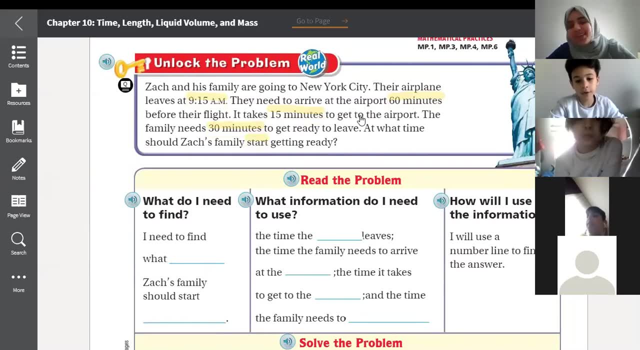 The number is 8 and 85 minutes. Okay, before you give me the final answer, tell me the step-by-step Example here, in the sentence The first time, 9.. I need to find what first of all, The start time, or the end time at that? 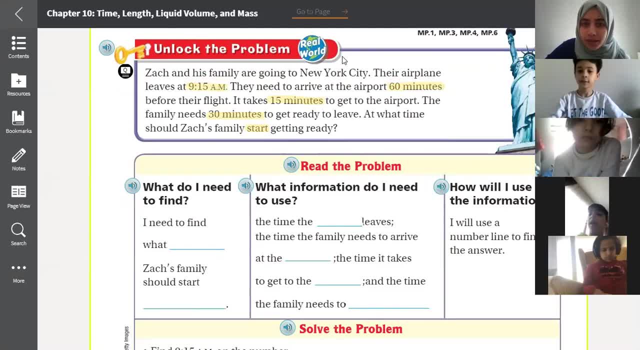 The end time. Okay, so are you sure? Look at the question again. Okay, so are you sure? Look at the question again. Okay, so are you sure. Look at the question again: At what time should Zack's family start getting ready? 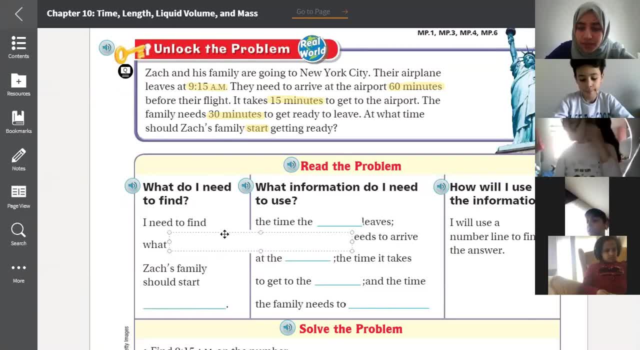 What do I need to find? Start or end time. Start, Start time, because they gave us the key word, So here I'm going to put start time. I need to get those for your guys to be able to read right. 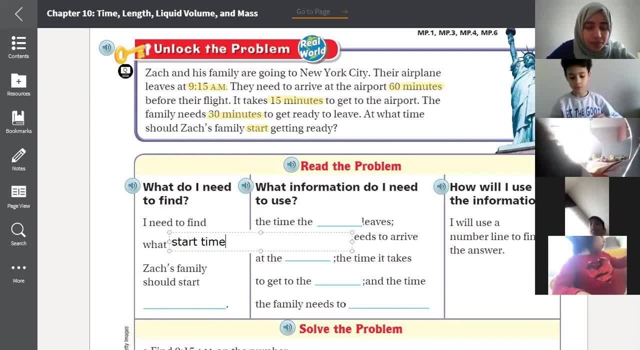 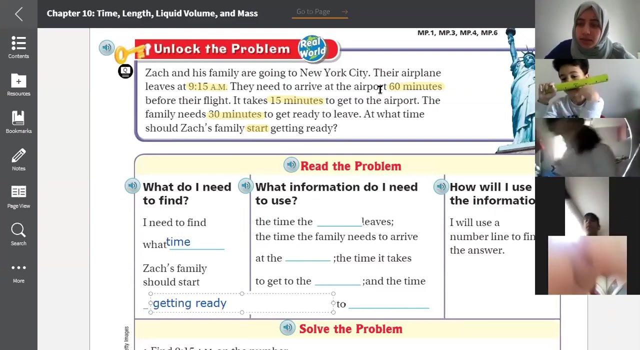 I need to get those for your guys to be able to read right, And Zach's family should start what They will travel, So they already gave us here something to start again. Time to start getting ready before they travel. For the next part. what information do I need to use? 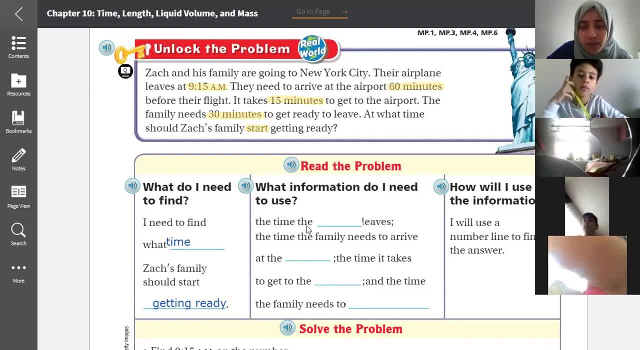 First of all, they gave us the time, the what leaves. Look at the question again: What is leaving? What is leaving at 9.15 am? Rana, 50,, no, 60 minutes. What's leaving at 9.15 am? 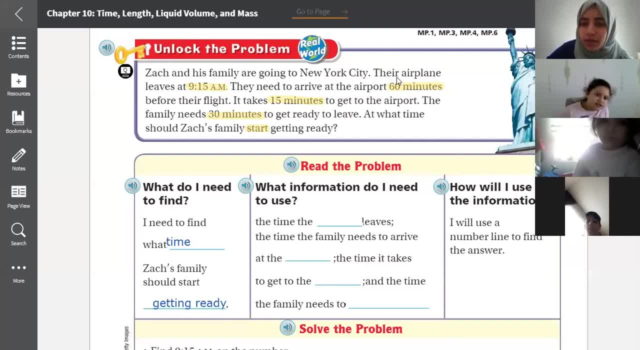 Read the sentence from here again: 9.15.. Okay, what's leaving at 9.15?? Read the sentence. Their Airplane Leaves At 9. 15 am- T A M. So what's leaving at 9.15 am? 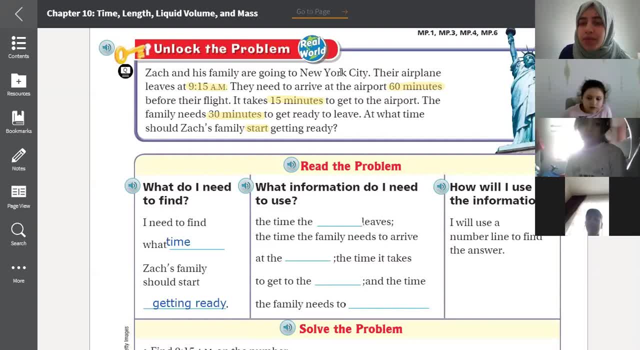 What's going to happen at 9.15 am? They said their airplane leaves at 9.15 am. So what's going to happen at 9.15 am? What's leaving? The airplane Rana is going to start moving at 9.15.. 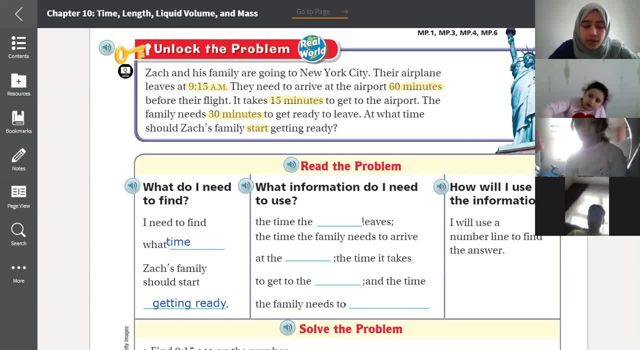 So we need to write that the airplane leaves at 9.15.. Okay, The airplane. Can you repeat that? The time that airplane leaves? Okay, so this is when the airplane is going to leave: 9.15.. And the time the family needs to arrive at the. so where do they need to arrive? 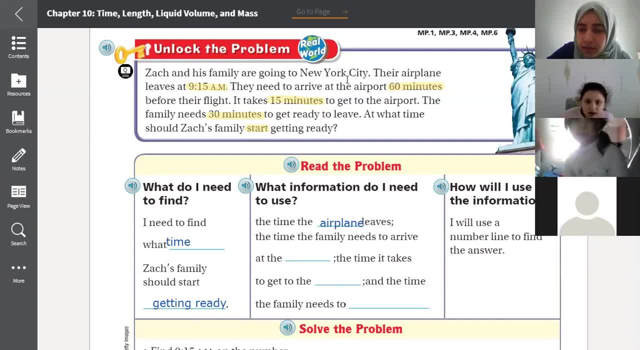 They need to arrive at At 6,- no, New York, Okay, but before 60 minutes- At the what Airplane Airport. It's the place where they need to get the ticket and put their luggage right, And the time it takes to get to the. 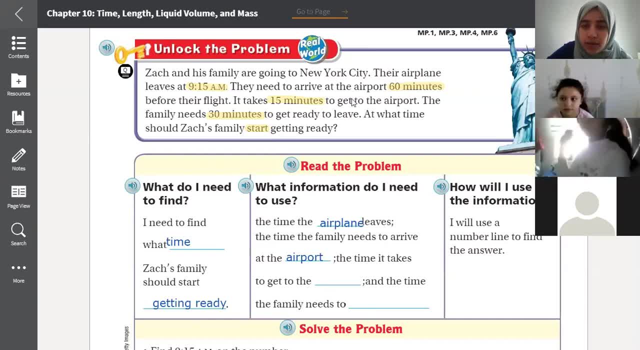 So they need to get to what. It takes 15 minutes to get to where Airport Airport. So again it's going to need 15 minutes to get to the airport. So we need to count all this time to calculate when the start time of them getting ready needs to be. 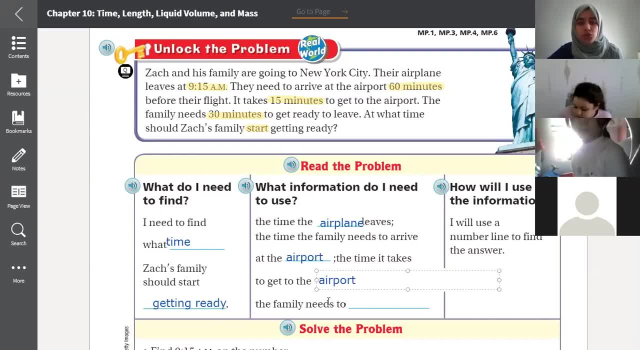 And the last one. the family needs two. What do they need? They need 30 minutes to do what? 30 minutes to To leave? They need 30 minutes to get ready to leave. Yes, good job, Get ready to leave. 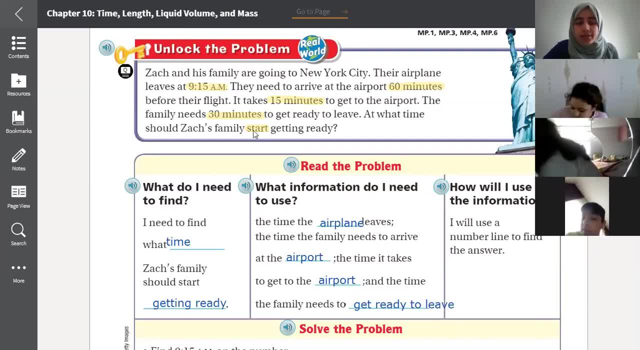 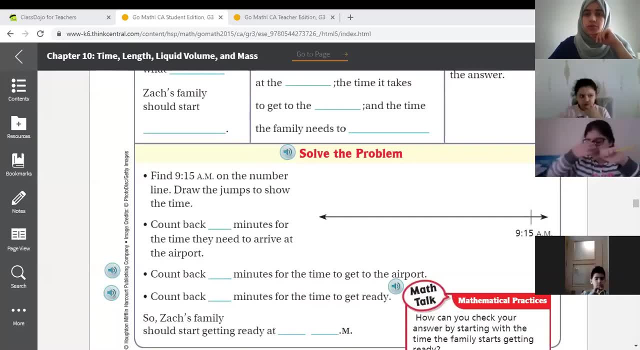 So we need to use this information to find the start time. Thank you, Rena. We're going to use a number line to solve the problem And look back at the information that was given to us So we know that the end time is 915.. 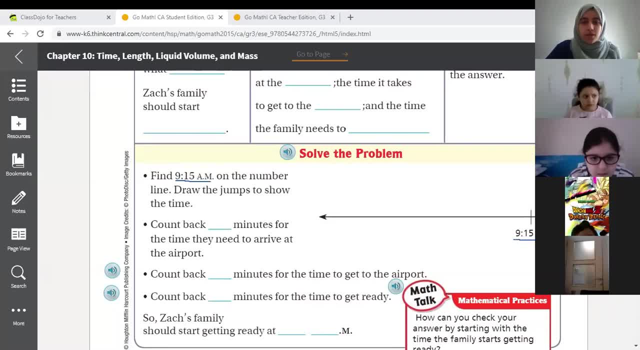 That's why we put 915 at the end of the number line And we need to draw jumps to show the time that we need to reach to the starting time. So first of all, we need to count back a few minutes for the time they need to arrive at the airport. 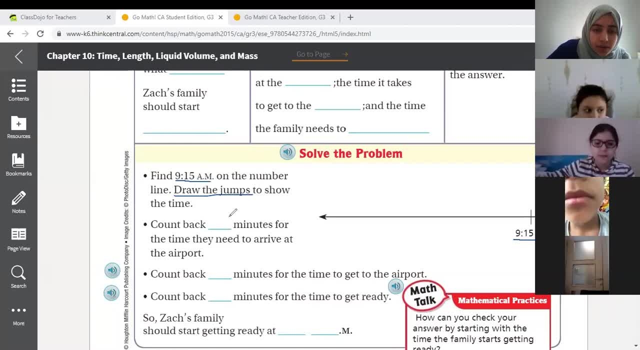 So they need to arrive 60 minutes to be in the airport. So first thing we're going to do is we're going to count back by 10. And then we're going to count back again, because for the time to get to the airport it was 15 minutes. 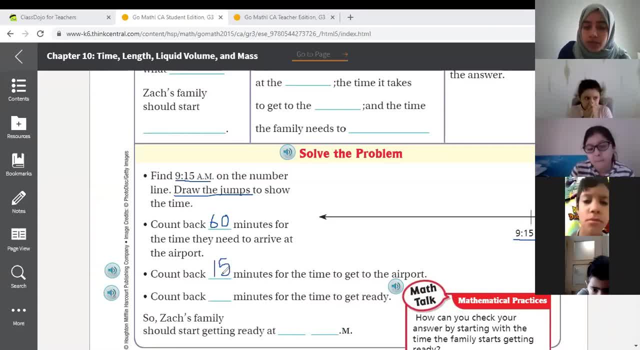 We know that time to get to the airport was 15 minutes And the time for them to get ready was 15 minutes And the time for them to arrive was 30 minutes. So we need to count back by all these minutes to reach to the start point. 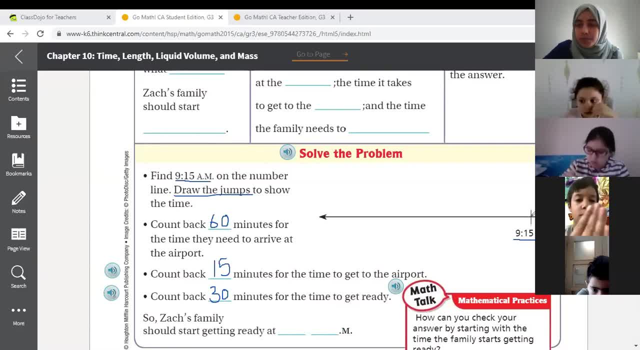 So we can start counting back by 10.. Let's start counting back by 10.. So I'm going to count back by 10.. So it's going to be minus 10 minutes And then keep doing it until it's 60.. 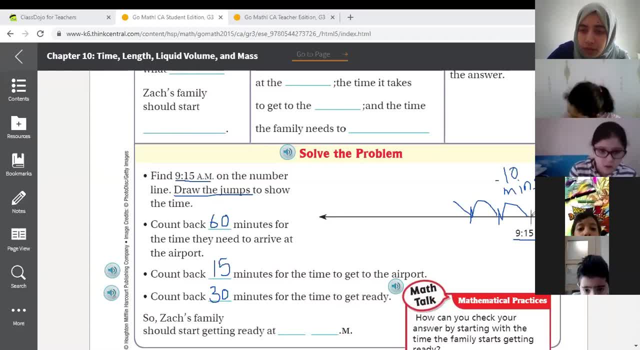 So 20,, 30,, 40,, 50,, 60. So minus 10.. I'm going to try to make it as clear as possible: 20,, 30,, 40,, 50., 60. And then again let's see how much time it's going to be here. 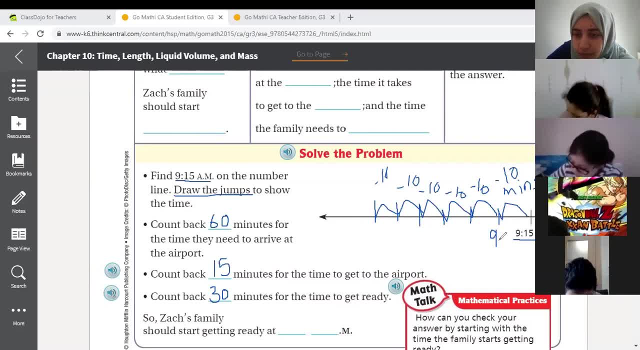 So we know 15 minus 10 is 5.. So it's going to be 5 minutes after 9.. And then minus 10, it's going to be a new hour. 9 minus 1 is 8. And the minutes is going to be 55.. 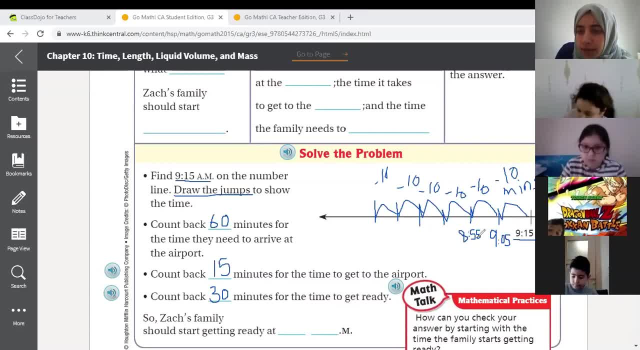 Because 10 minus 5 minus 5 will be 9, exactly. And then another time we need to subtract by 5.. Because in total it's 10.. It's going to be 8.55.. We need to subtract again by 10.. 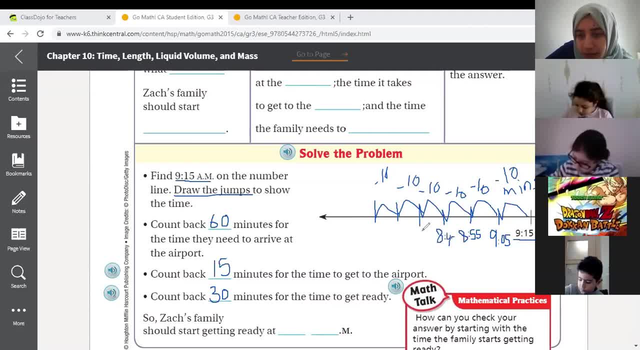 And it will be 45 minutes after 8.. 35 minutes after 8.. Try to make your handwriting small and neat. 25 minutes after 8.. 15 minutes after 8.. And now we're going to subtract the time that the family needs to get to the airport or to reach the airport. 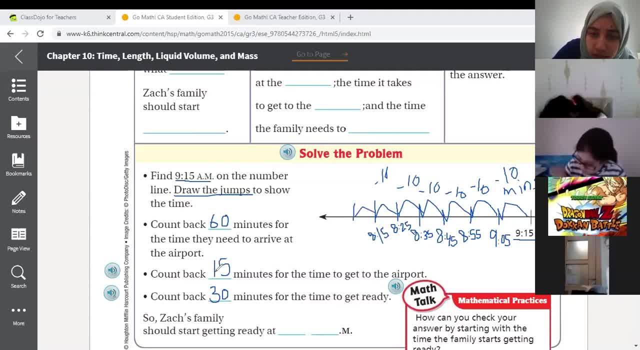 So it's going to be minus 15.. And we know that 15 minus 15 is 0.. So the time is going to be exactly 8 o'clock, And then the last thing we need to do is subtract by 30 minutes. 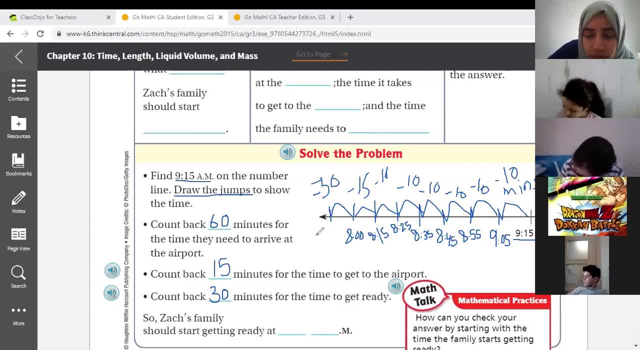 30. So we need to go down an hour 8 minus 1. And subtract 30 minutes, So the timing here will be 7.30.. So this is where we finish, because we subtract all the elapsed time. Zainab, after we subtract the elapsed time, what is the time that we reached at the end? 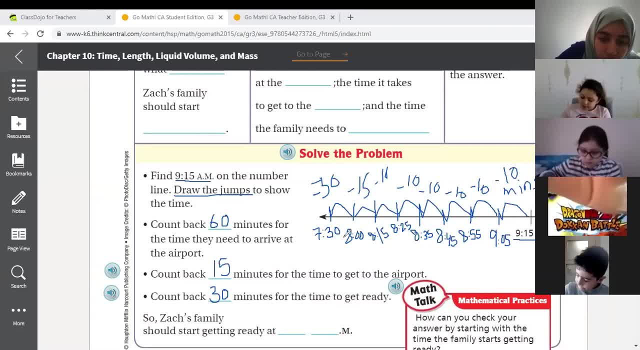 7.30 minutes 7.30.. So our starting time will be 7.30.. And is it am or pm? Am, Yes, am, So it's still am, Because it didn't skip midnight. 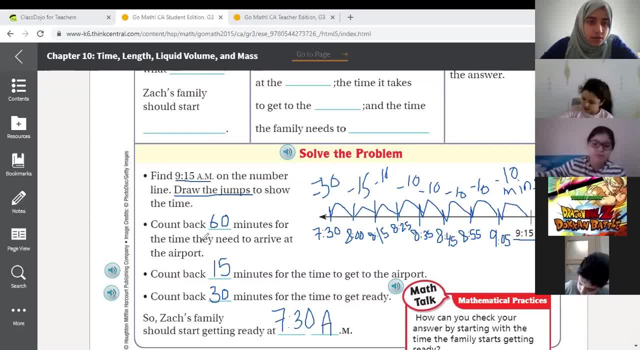 Good job, Zainab. So notice here how, first of all, we need to find all the minutes in between- That represents the elapsed time, And then we also need to count back. if the end time was given And if they gave us the start time in the beginning, we need to count forward. 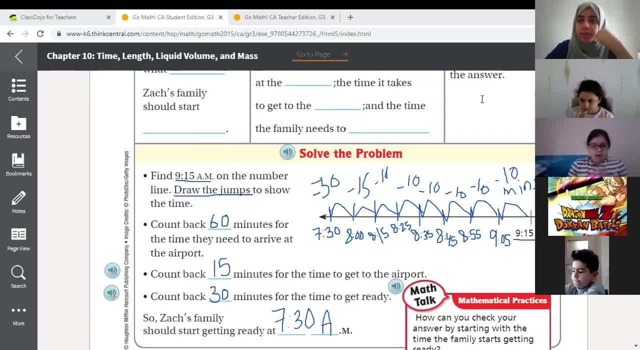 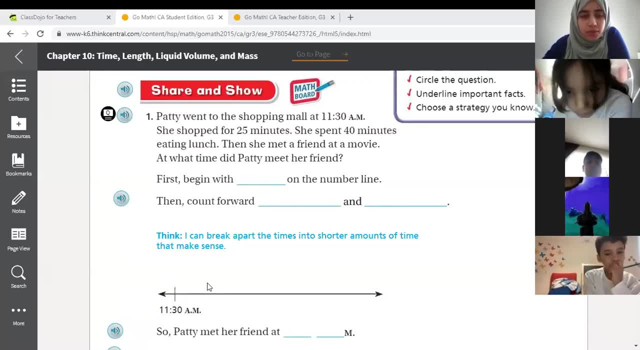 I'm going to give you guys a second to write the number line And, Yamin, I'm going to write the answers above it so you can have a chance to copy it. Read number one, please. Patty went to the shopping mall at 11 and a half am. 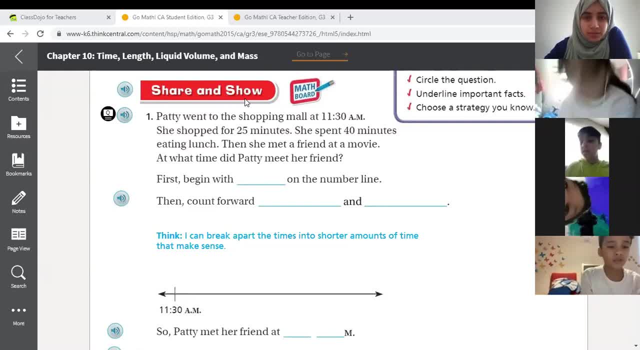 She shopped for 25 minutes. She spent 40 minutes eating lunch. Then she met a friend at a movie. At what time did Patty meet her friend? Thank you, Izan. So here they're asking for the time she met her friend. 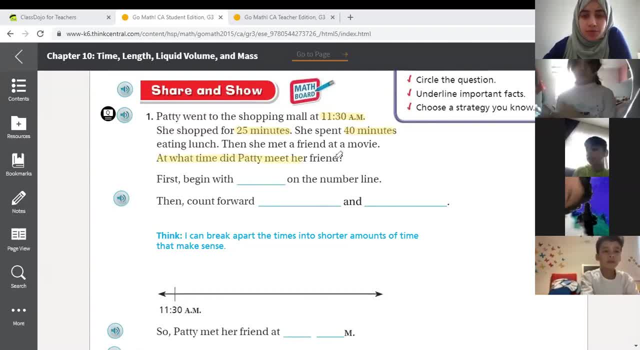 Is this the start time or the end time that they're asking for? So she went to the mall at 11.30 am. So she started her trip and went to the mall at 11.30 am, Or 30 minutes after 11.. 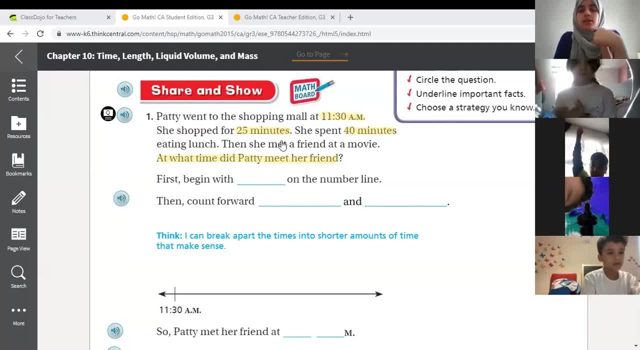 She shopped for 25 minutes. She spent 40 minutes eating her lunch. Then the last thing she did was meet her friend. So when they ask us: what time did she meet her friend? Are they asking for the start time or the end time? 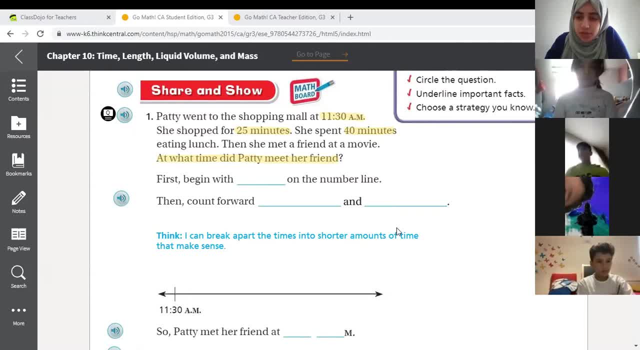 Is this the last thing she did Or the first thing she did when she met her friend? Last thing, Last thing. So it would be the end time that we need to find correct. Mm-hmm. Okay, Thank you, Izan. 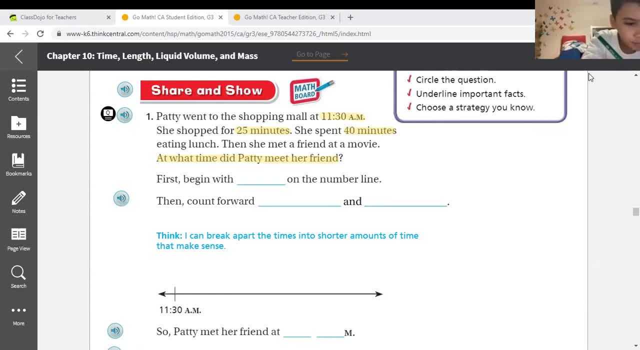 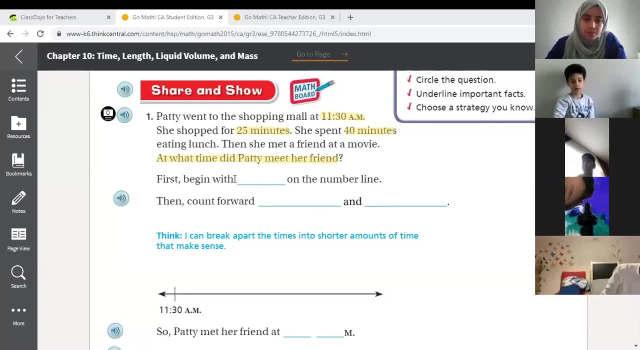 Fahad. Yes, So first begin with. what do we start with? on the number line, What time did they give us Fahad? 11.30 am. Good job, They gave us the start time, which is 11.30 am. 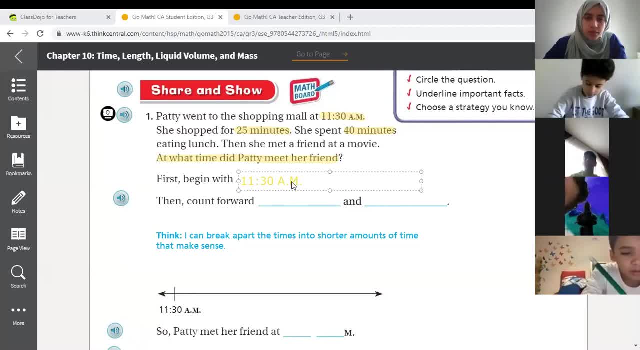 So we need to start our number line with 11.30 am And then we need to count backwards or forwards, Because we have the start time. do we need to count backwards or forwards? Forwards, Forwards, Excellent. So we need to count. 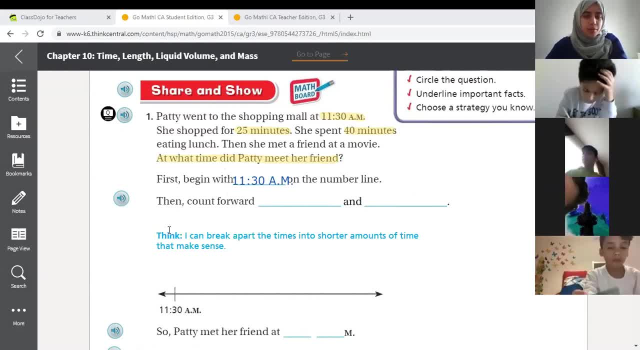 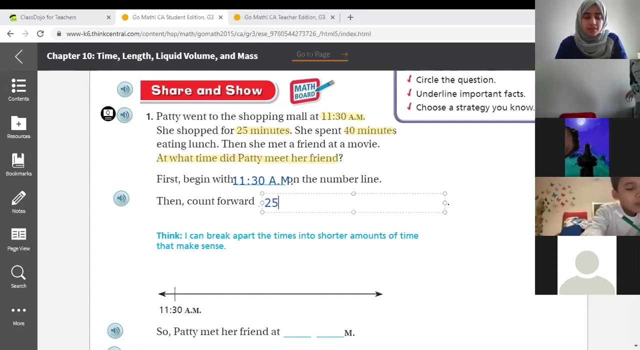 Thank you, Fahad Asil. How many minutes do we need to count forwards? Look at the minutes I highlighted in the question, Asil. How many minutes do I need to count forwards? 25.. 25 and 40.. 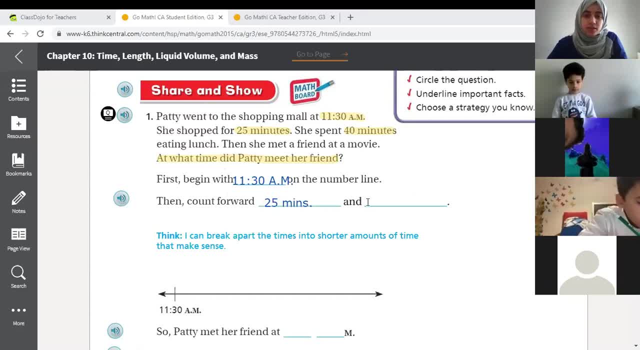 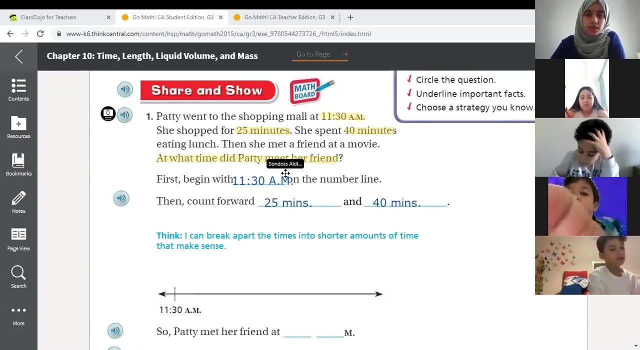 40. Excellent. So we have 25 and 40 minutes, which are the elapsed time or the time spent during this activity. So I'm going to start counting up here. So I'm going to start counting up by 10.. Yusuf, when I start counting up by 10 here, 11.30 will become. 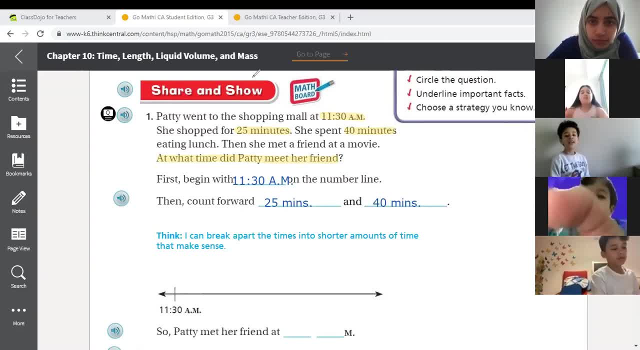 Um, So I'm adding by 10. Plus 10 minutes. Okay, 11.30? Will become what? So 30 plus 10? 40., 40. So I will have 40 minutes after 11. And I need to count again up by 10.. 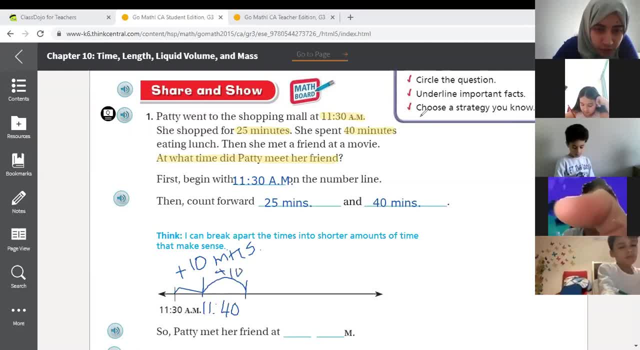 So plus 10.. 11.40 will become What's 40 plus 10? 50. 50.. And I need to count now by 5. Because I have 20 minutes in the tens place. So I counted by 10 and then 20.. 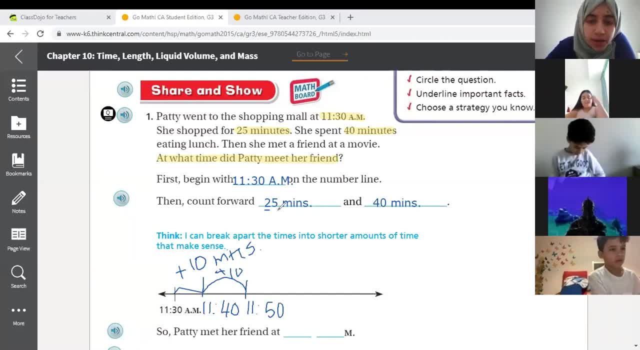 10 plus 10 is 20.. And now I need to count up by 5 in the ones place. So when I count up by 5. 11.50 will become what? 50 plus 5? 55., 55.. 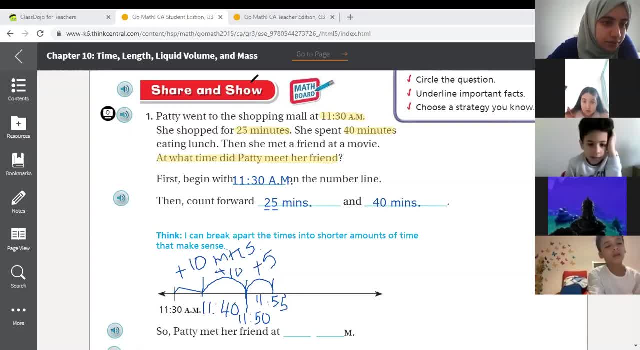 Yes, Good job. Thank you, Yusuf Zaina, your turn. So now that I finished counting by 25.. I need to start counting by 40 minutes, right? So when I count up here, I need to count how many times by 10?? 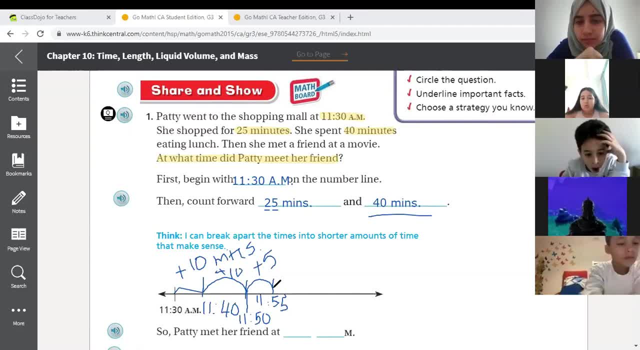 How many tens do I have in 40?? Look at the tens place. How many tens? Four tens. So I have four tens. So I need to count by 10 four times. So one, Two, Three And four, right? 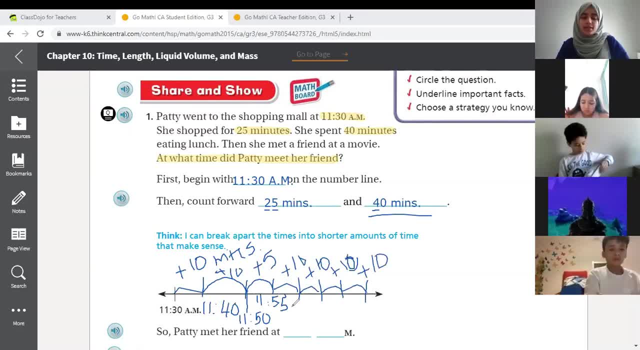 So from 11.55.. When I add 10 to 11.55.. What do you think the next time will be? I know 11.55 plus 5 is how much It's 12 and 5 minutes Exactly.